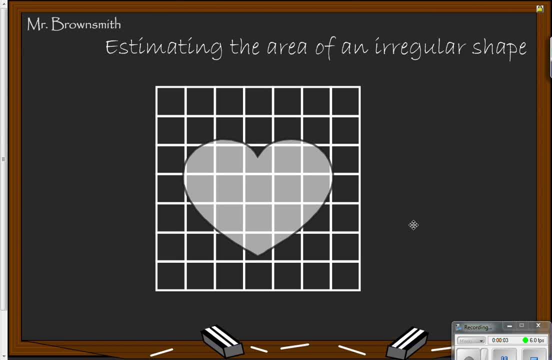 Today I want to talk about how to estimate the area of an irregular shape using a grid in the back to help me figure out the full area of this, or close to the full area of this. So the first thing that I like to do is to count all of the full squares that we've got in the figure. 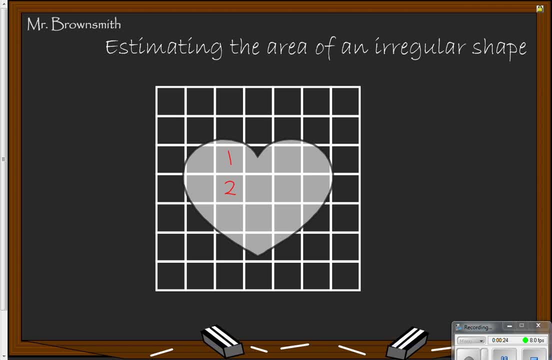 So, for example, we've got one here, here's another one, and I'm just going to mark them with numbers so I don't lose. count One, two, three, four, five, and it looks like we've got a six here. 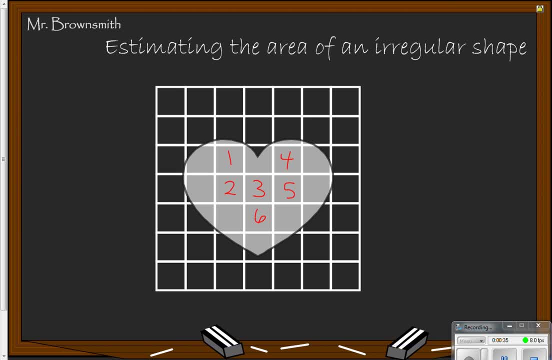 I've got some that are pretty close and we're going to get to those in just a second. So, after I've counted my full squares, what I'm looking to do is trying to find partial squares that only need another partial bit to make them full. 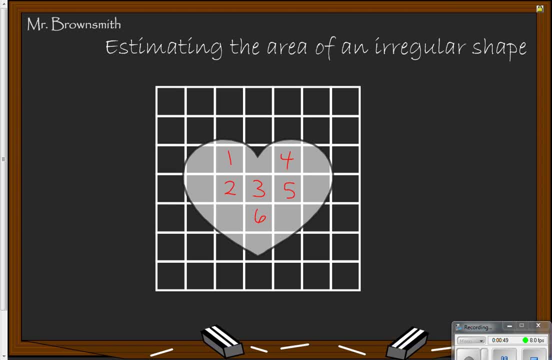 For example, if I look at this one right here, this little tiny guy maybe right here, you can see I've got that little section right there And I've got this one right here. that's kind of missing a section very close to that amount. 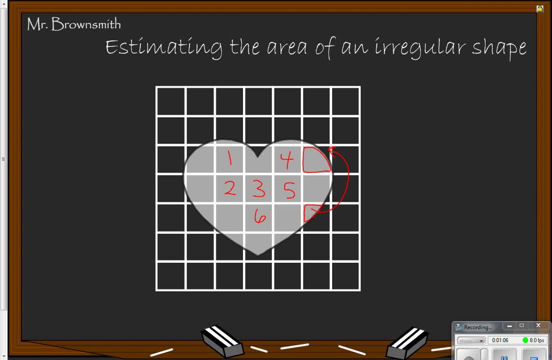 So if I took this piece right here and maybe added it, I'd probably get a full square. So that's what I'm looking to do is to find partial squares that, when added together, are going to give me close to a full one. And here's another example. 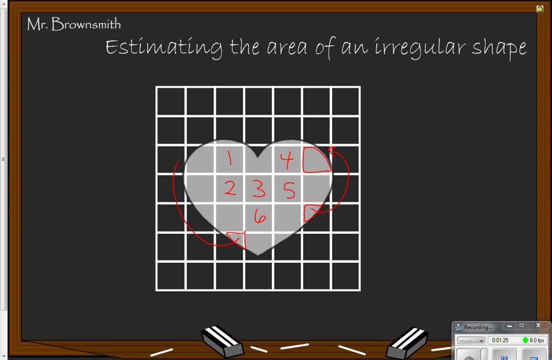 I've got a little section right here and maybe if I added that little section up here to this one, that would give me a full one. So already right here, with these ones right here and right here, I probably now have about seven squares. 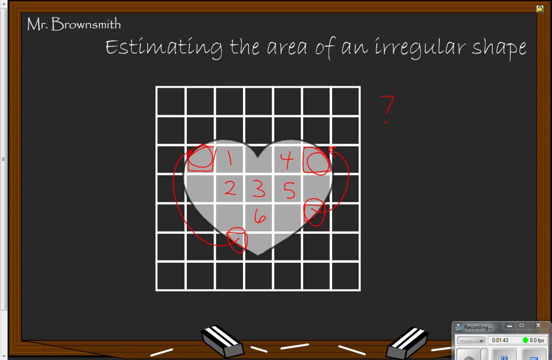 And then this one here and this one here. that probably gives me about eight, And now I'm just looking for other ones that I can piece together to give me. So I've got this one right here and maybe this one right here, So that might give me nine.